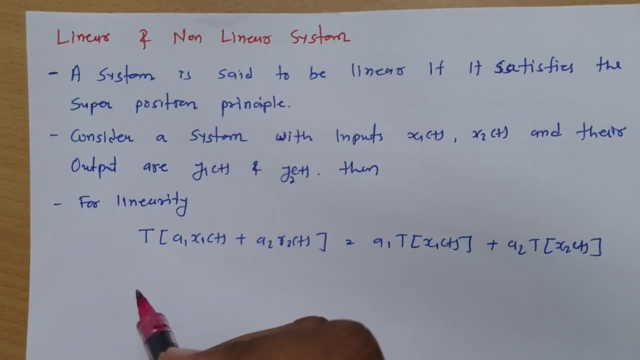 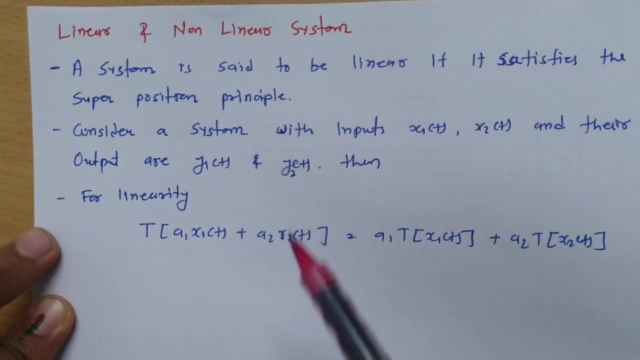 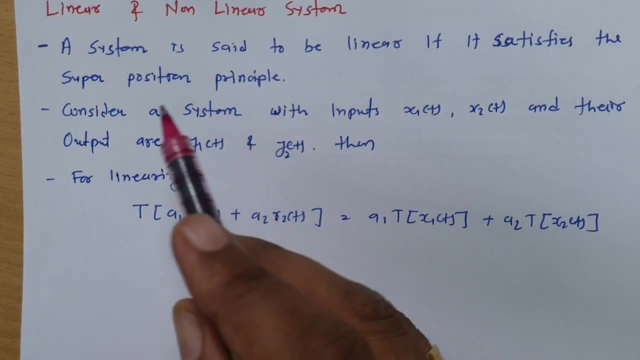 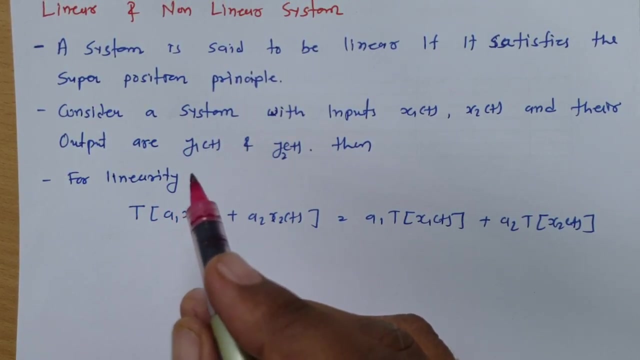 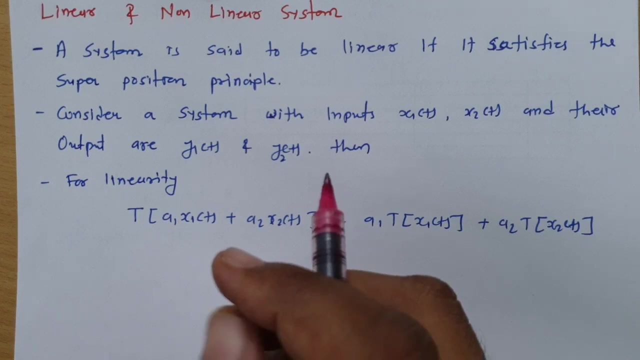 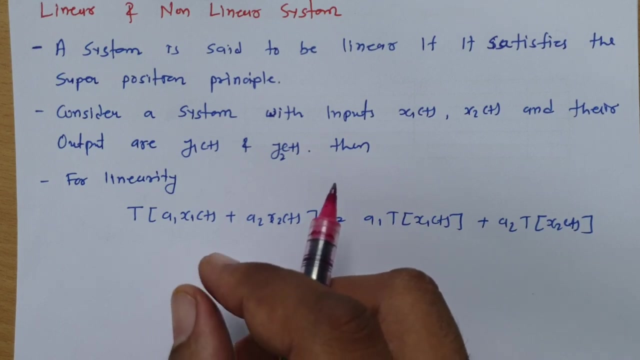 Welcome to signal and system lecture series. In this session I'll be going to explain first classification of system, that is, linear and nonlinear system. So what is linear system? A system is said to be linear if it satisfies superposition principle. So what is superposition principle? Superposition principle is when you give different inputs and you take output, And if you combine those inputs and if you take output and if both are same, in that case one can say it is following superposition theorem. 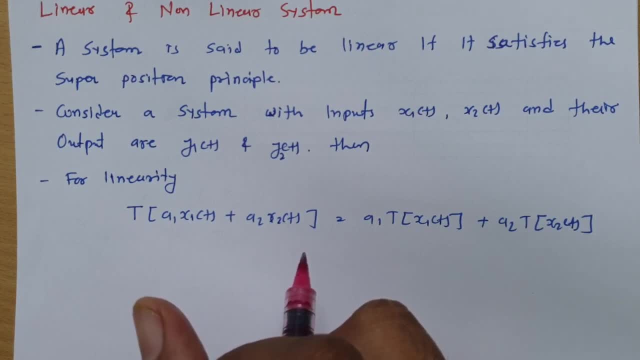 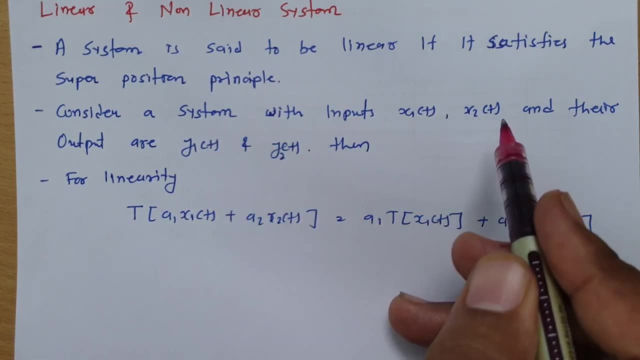 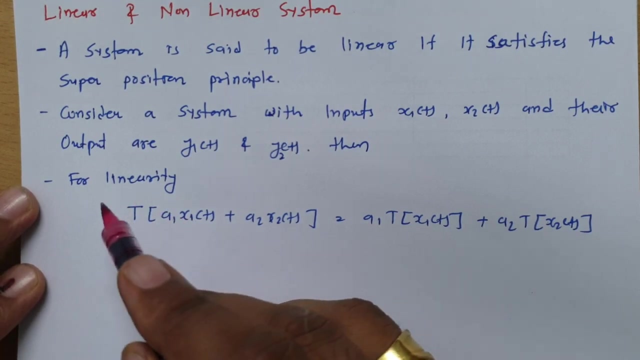 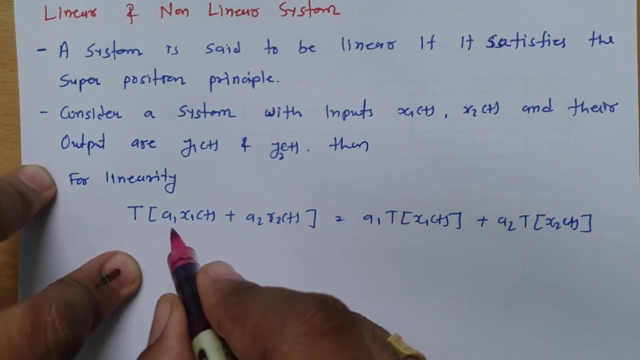 And that is what giving you, whether this given system is linear or not. So here I'm considering one system with input x1 t and x2 t, And in that case their outputs are y1 t and y2 t. So what will be linearity by superposition theorem? So see here this transpose of a1. 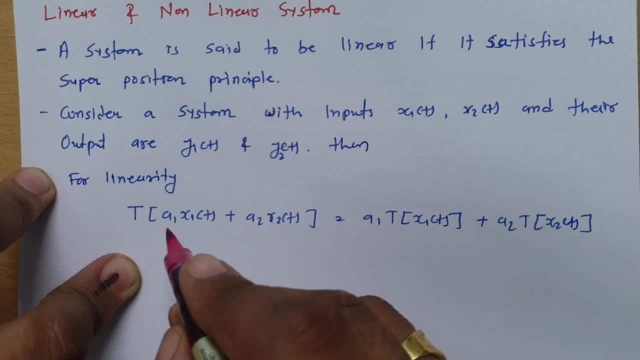 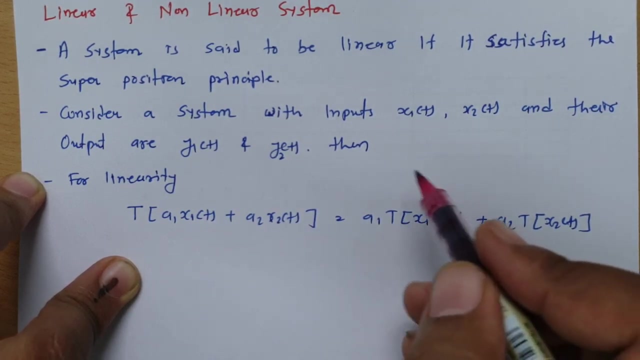 x1 t plus a2, x2 t. So that is what combined signal response Transpose of that is what actually response of system. Here I'm combining two signals, x1 t and x2 t, And here I'm taking response of system with just individual inputs. So see a1 transpose of x1 t, where here I have response of system with input x1 t and here I have response of system with x2 t and over here I have response of system with combined input. 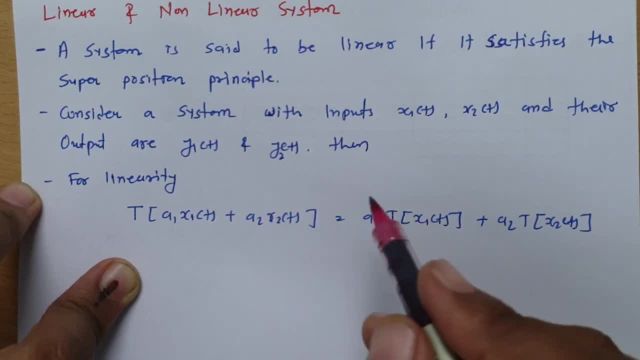 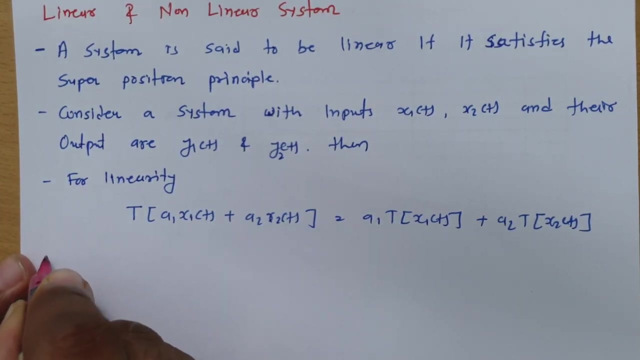 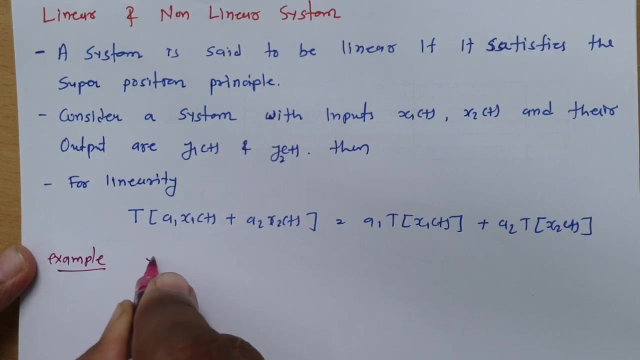 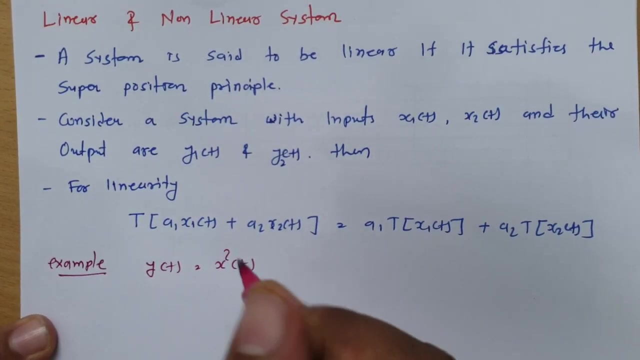 So if both are same, then one can say it is following superposition theorem And that results into linear system. So let us try to understand this with example, so it will be more clear. So for example, if I say I have input output relation, yt is equals to x2 t. 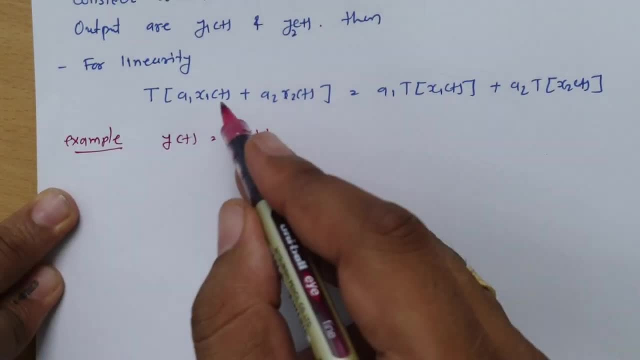 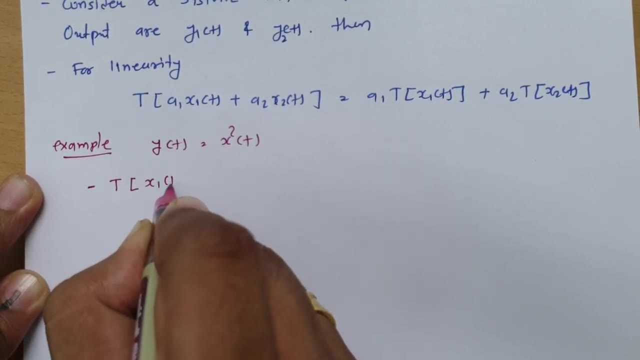 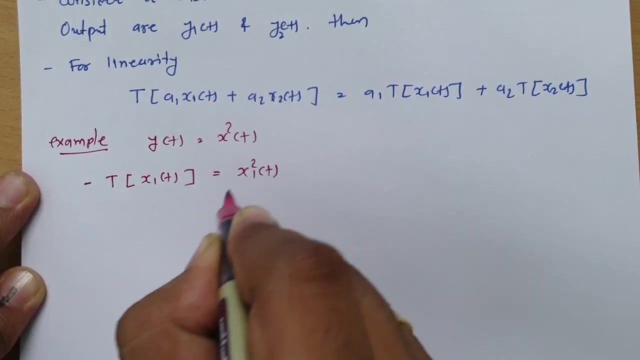 So in this case, let us apply this. So in this case, let us apply this. So in this case, let us apply this. So I shall see this condition. So if I calculate response of system with given input, x1 t, So that has to be x1 square t. 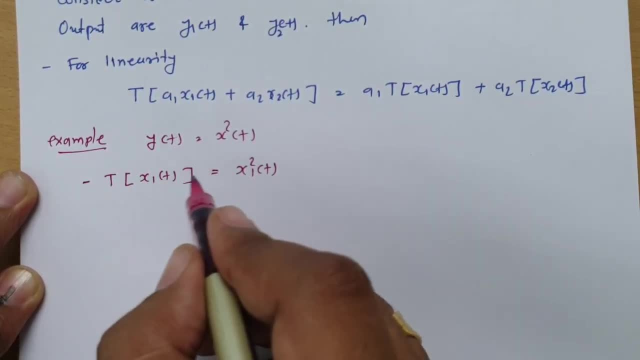 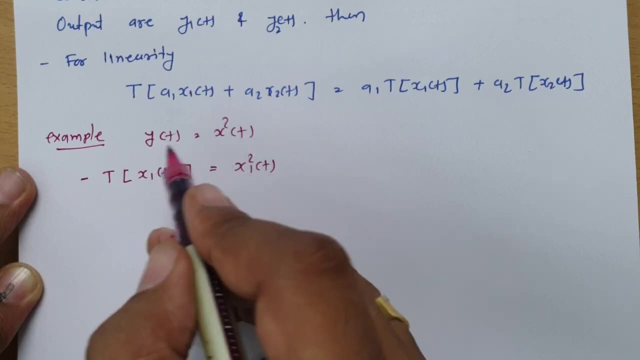 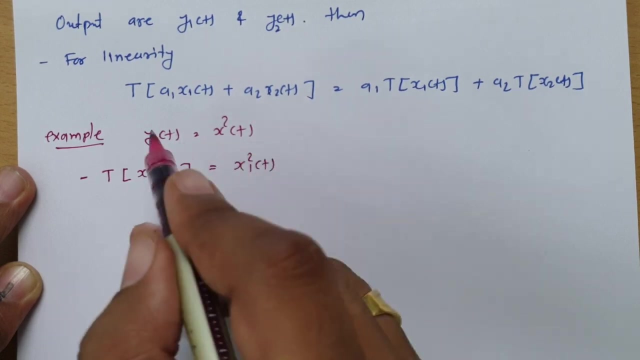 What is response? it is output. so transpose of x1 means output, with input is x1 t. So here, as we know, relation of input, output is yt equals to x2 t. So transpose of x1 t, that will be x1 square t as per this relation, and if you apply input x2t, so transpose of x2t. 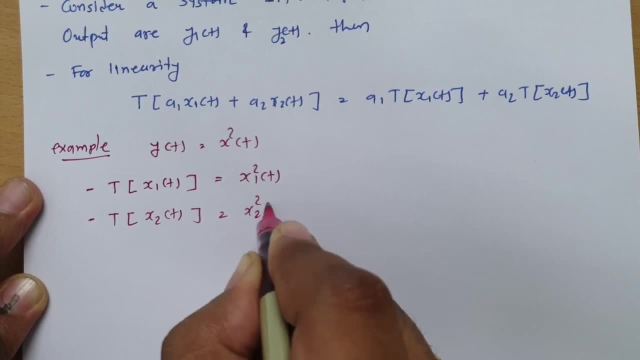 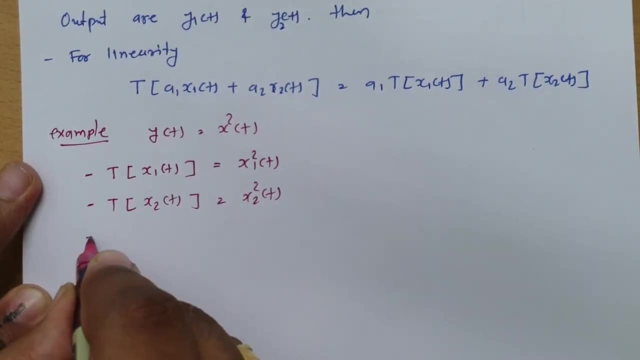 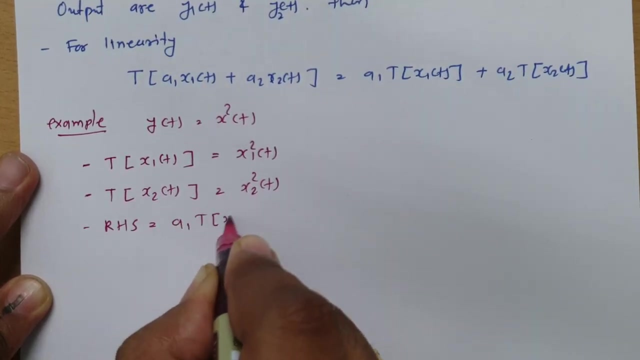 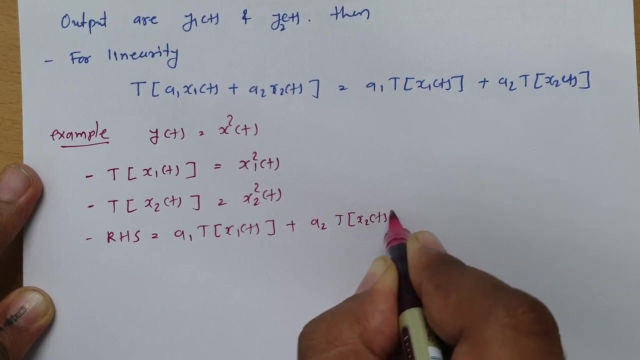 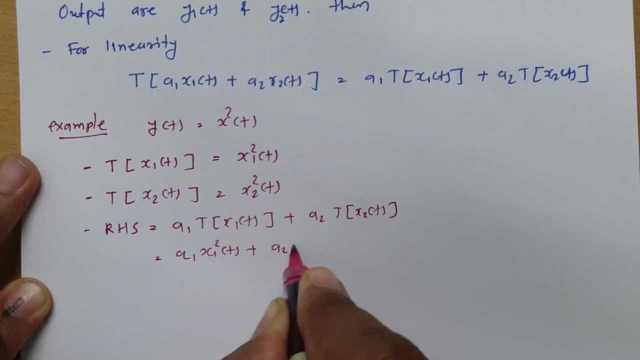 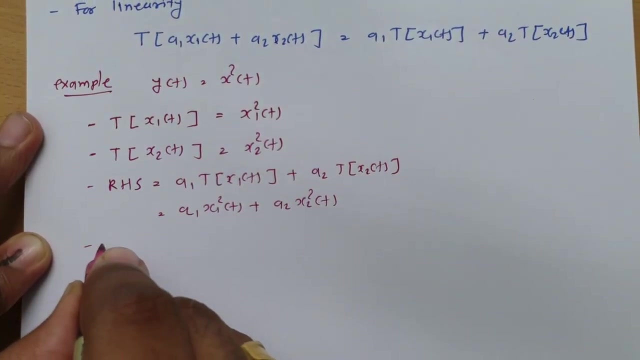 so that has to be x2 square t as per this relation. So if you calculate RHS, so RHS of that that has to be a1 transpose of x1 t plus a2 transpose of x2 t, so that will be a1 x1 square t plus a2 x2 square t. Now if we calculate LHS, then LHS is what LHS is. 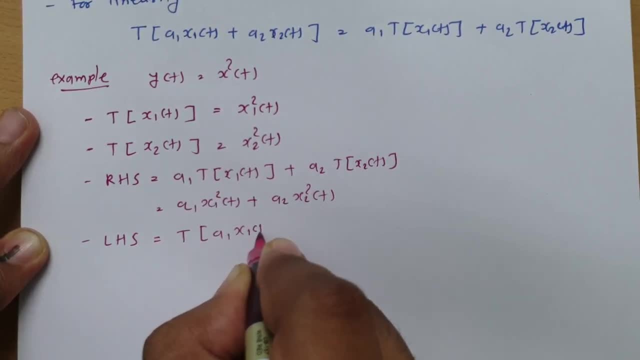 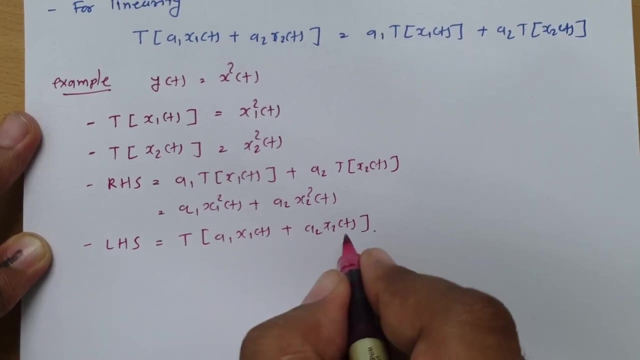 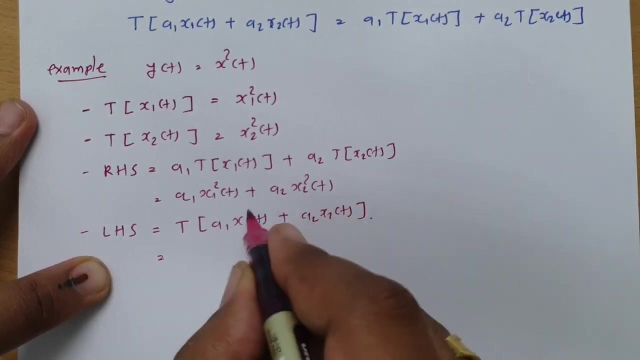 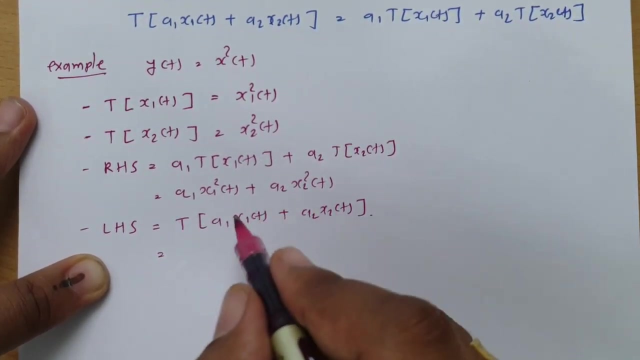 transpose of a1, x1 t plus a2, x2 t. so now we are combining this two signal, x1 t and x2 t. so if you calculate this response output, so that will be square of this input. as this relation is, yt is equals to x square t, so response of this will be square of this given input. so if you do, 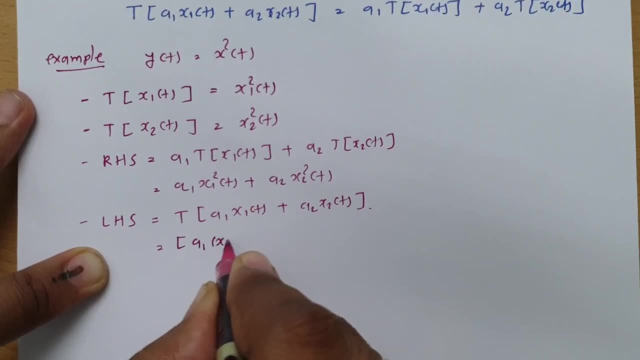 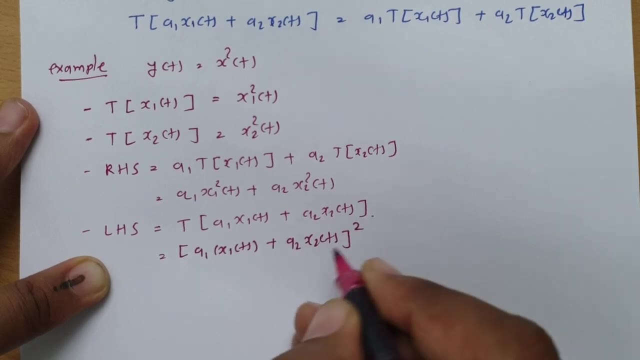 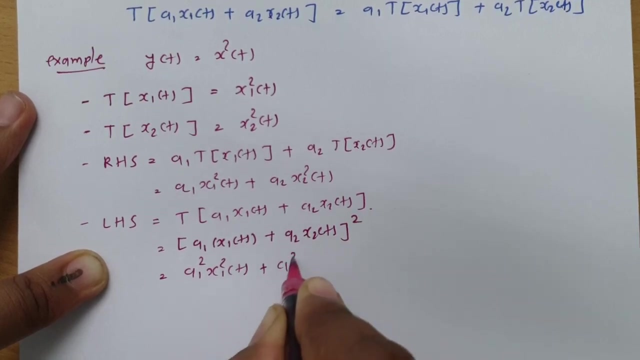 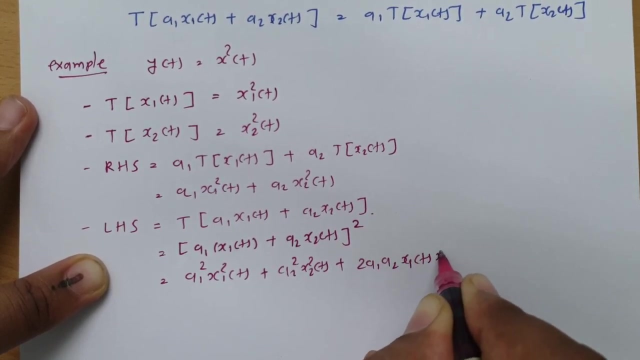 squaring of this input: a1 x1 t plus a2 x2 t square, so that will be a1 square x1 square t plus a2 square, x2 square t plus 2: a1, a2, x1 t, x2 t. so this is not actually. 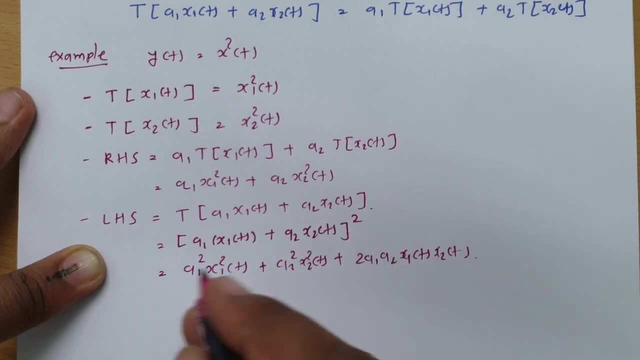 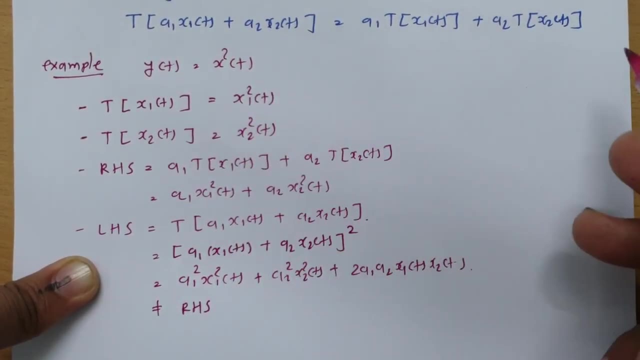 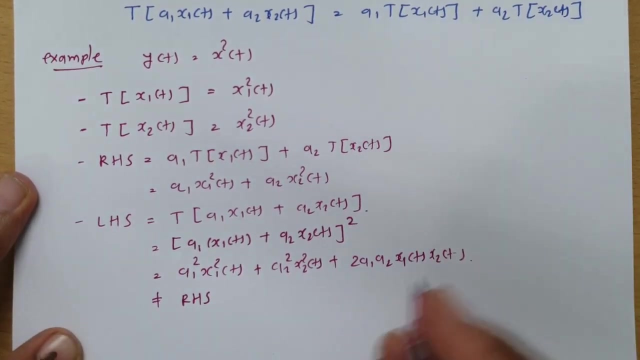 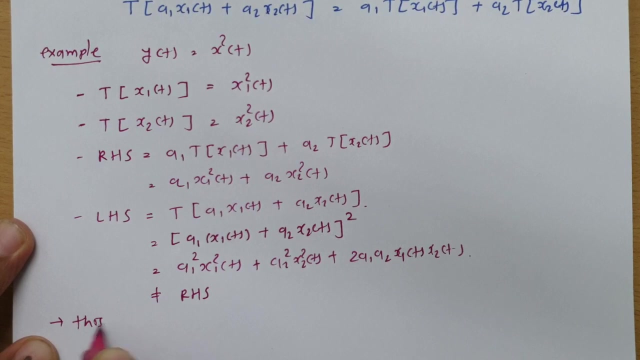 equals to x2 t, right hand side, which we have calculated. so this is not. equals to rhs means it is not following this linearity condition. so we can say this given system is non-linear system as it is not following principle of superposition, so this is non-linear. 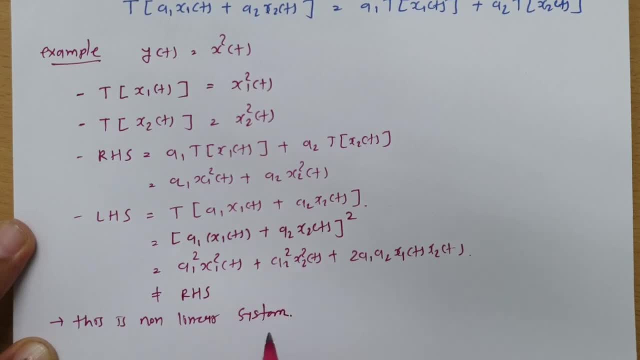 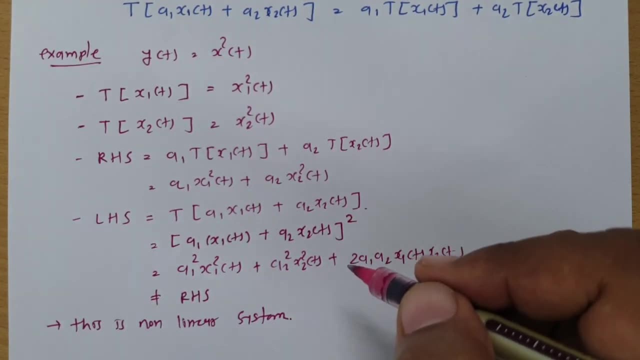 linear system as it does, it does not follows principle of superposition theorem. let us have one more example so it will be more clear. so if I give you one more problem, IF I say input y is equals to x2, so let us calculate response. if input is xt, transpose m is greater than this. the. 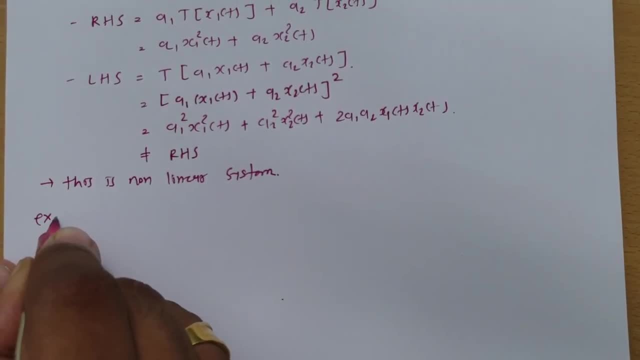 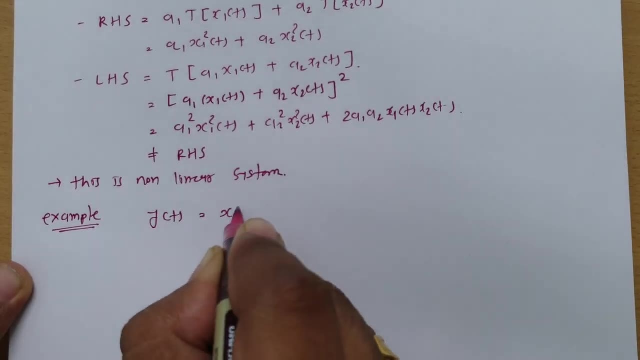 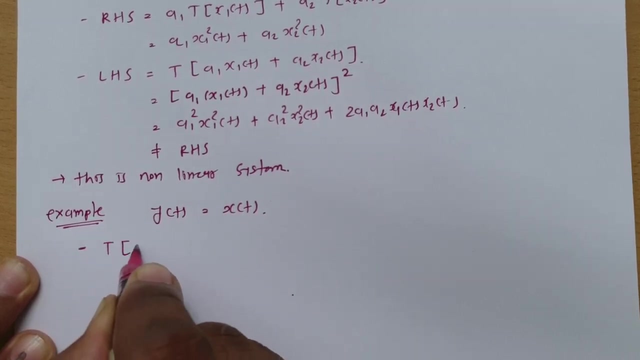 more here 不 Prof seconds f, my inputpedal. one more problem: f. by simple imput yt is equal to 2, agreement x in比 fp. let us calculate response if the input is x1t. so transposing of this result, ft, which we have calculated, this is 1 if the input is Mistate. 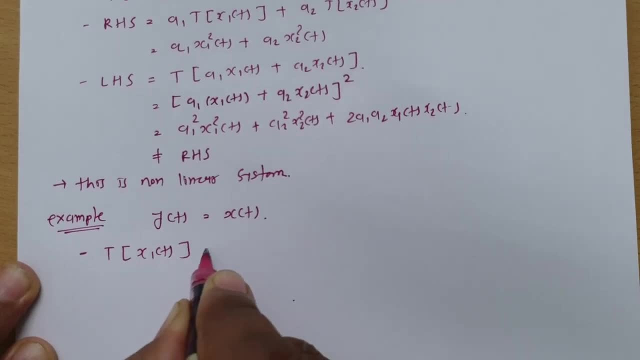 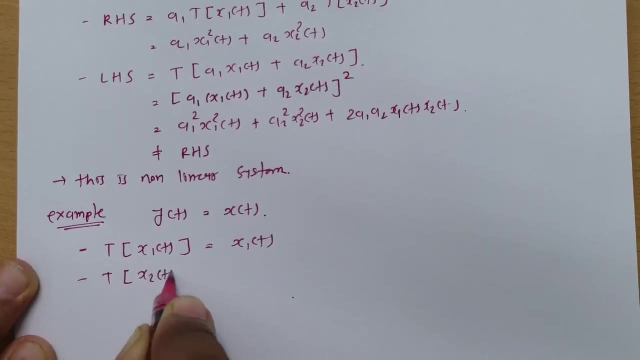 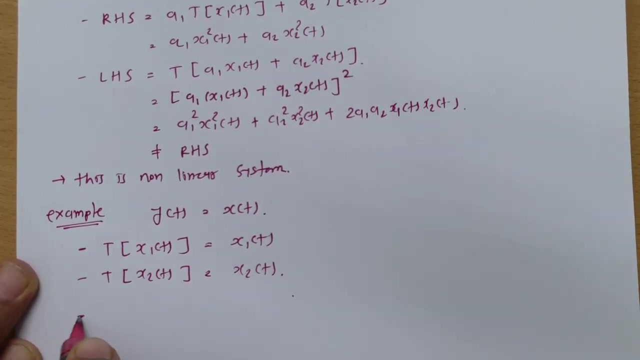 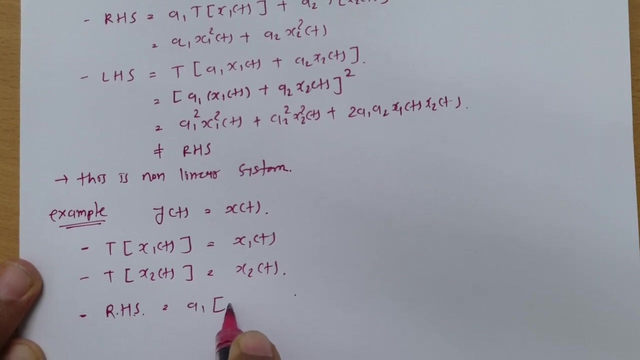 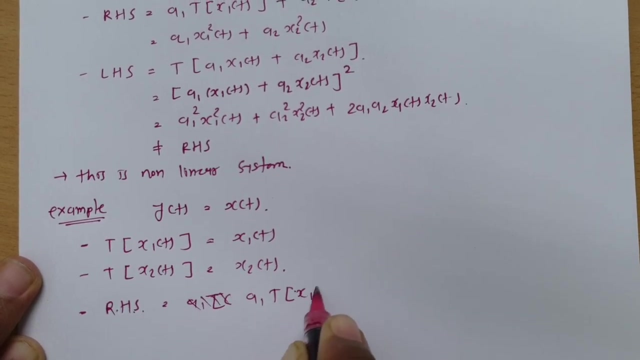 inline. So transpose of x1 t. so that is only x1 t. and if you calculate response of system with input x2 t, so that has to be having output, that is x2 t. So if you calculate right hand side, that is A1. transpose of A1. transpose of x1 t plus. 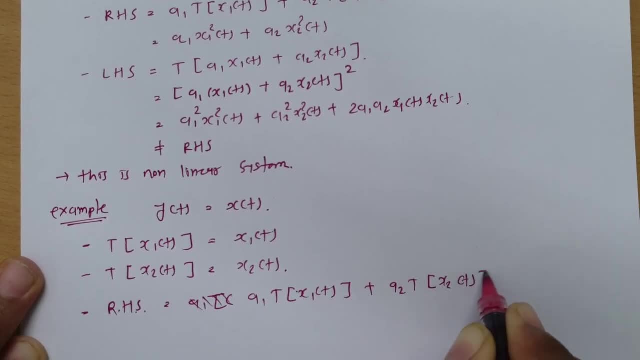 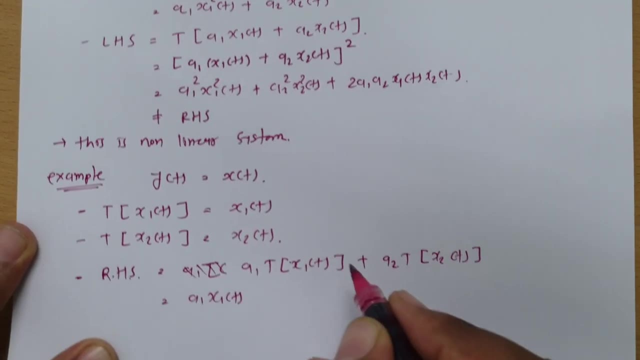 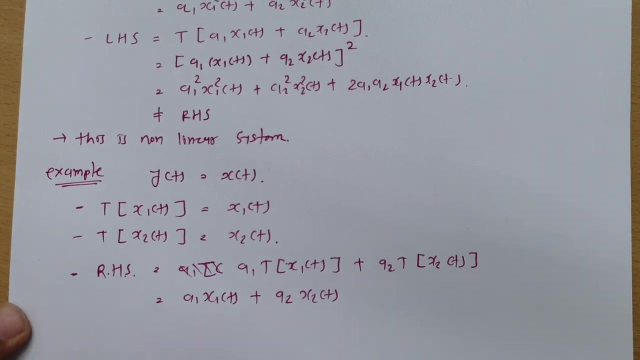 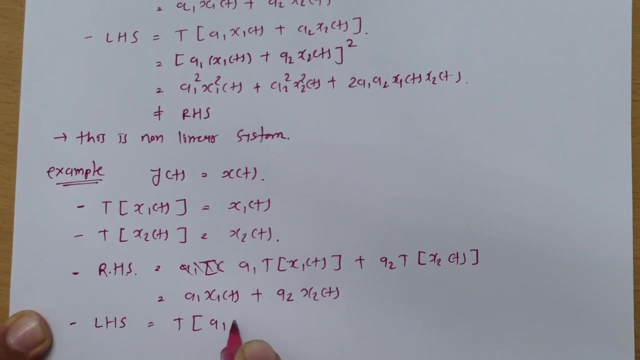 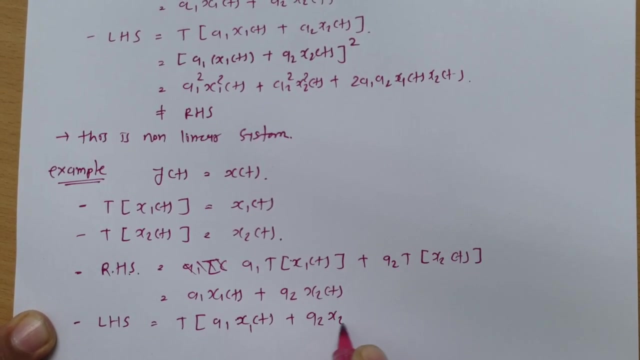 A2 transpose of x2 t. So that will be A1- x1 t- you can apply this over here- Plus A2 transpose of x2 t. Now let us have LHS calculation. So LHS is what Transpose of A1- x1 t plus A2 x2 t. 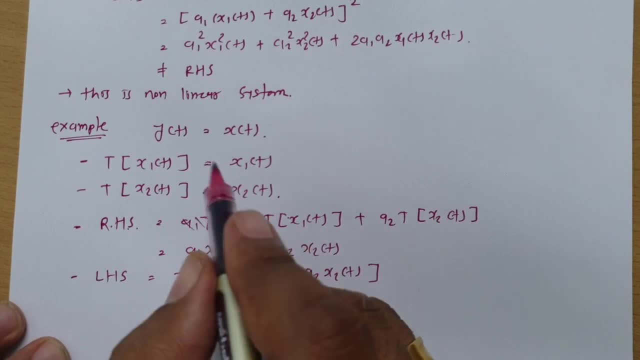 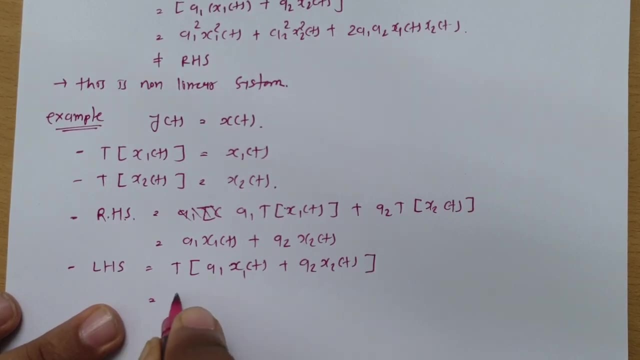 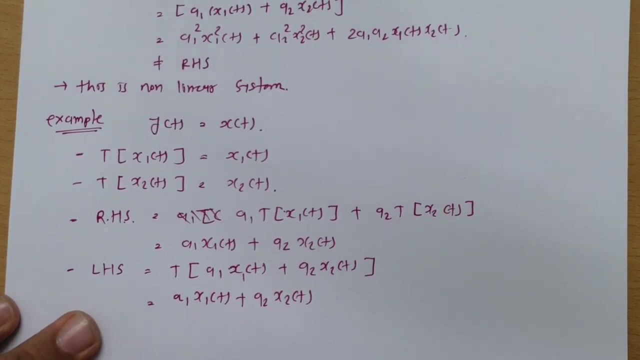 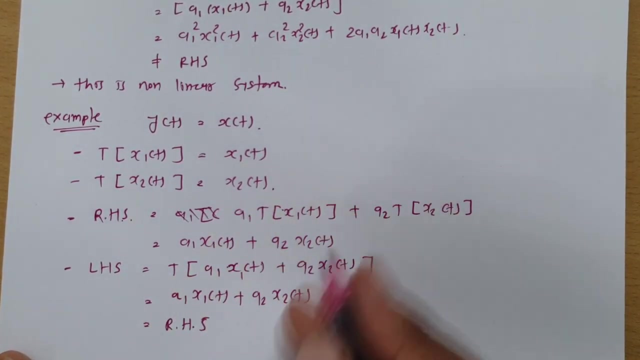 So in this case, as per this relation response output, that will be this: as yt is equals to xt, So over here this will be A1 x1 t plus A2 x2 t. So this is equals to right hand side. So one can say it is following superposition theorem. so this system is linear system. 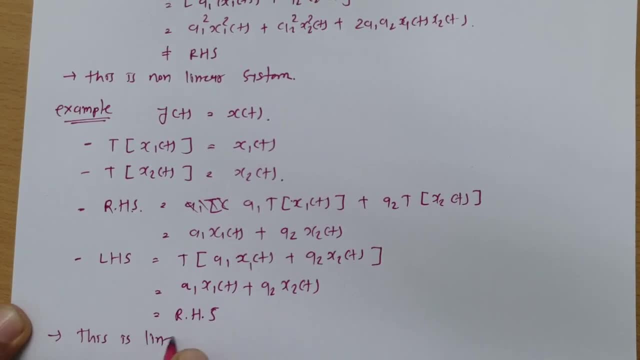 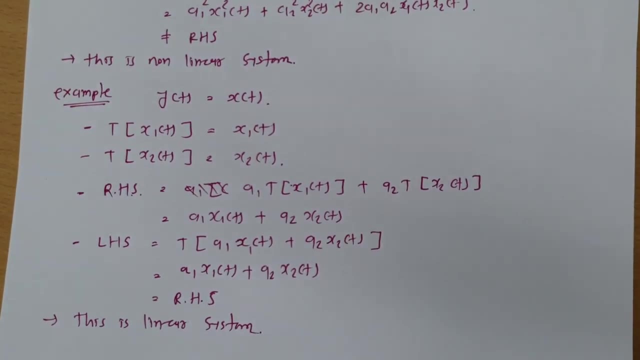 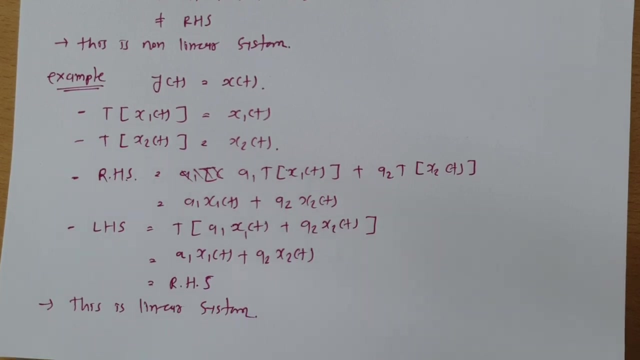 So this is linear system. So ultimately we can say: superposition theorem. So this is linear system, So this is linear system. System is said to be linear system if it is following superposition theorem. What is superposition theorem? Superposition theorem is explaining response of system with